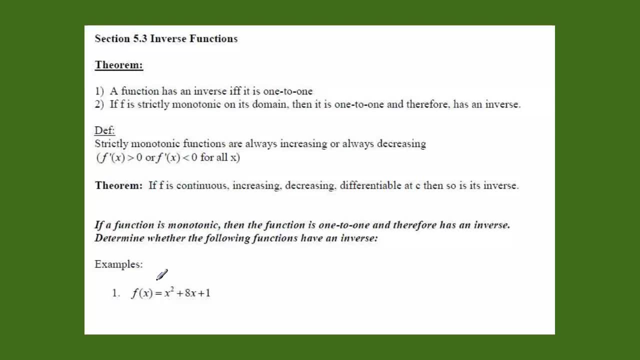 Okay, so for this video we're just going to be looking at how to determine whether or not a function has an inverse or not. Okay, so we have a couple of theorems in this section. The first one says that a function has an inverse if, and only if, it is 1 to 1.. Okay, so you already knew that If you have a 1 to 1 function, that tells us that you do have an inverse, and then vice versa, If you have an inverse, then that function is 1 to 1.. And remember, for 1 to 1, that is when your function will pass both the horizontal and the vertical line test. 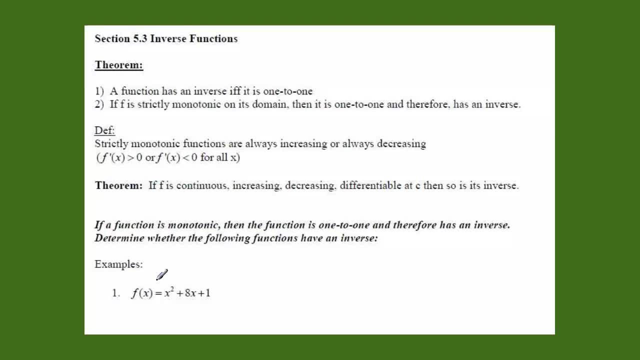 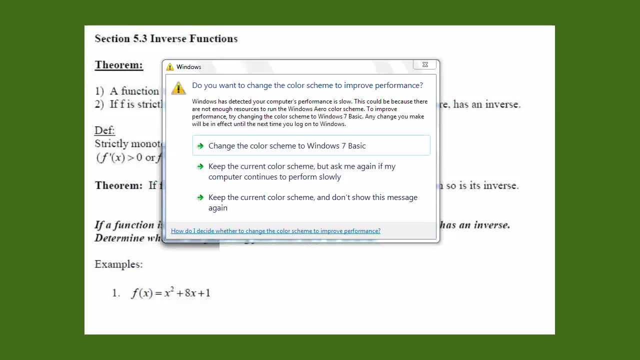 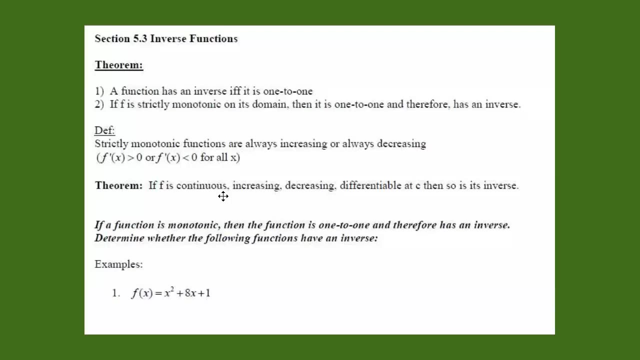 Okay, theorem 2 says if f is strictly monotonic on its domain, then it is 1 to 1 and therefore has an inverse. Okay, so our definition for a monotonic function is that a monotonic function is just a function that is always increasing or always decreasing. So that means that on a particular interval f prime will always be positive or f prime will always be negative. 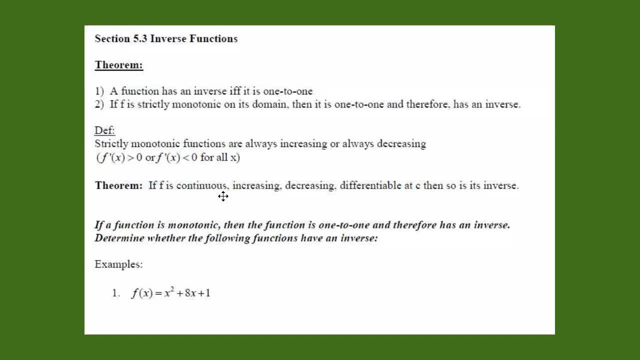 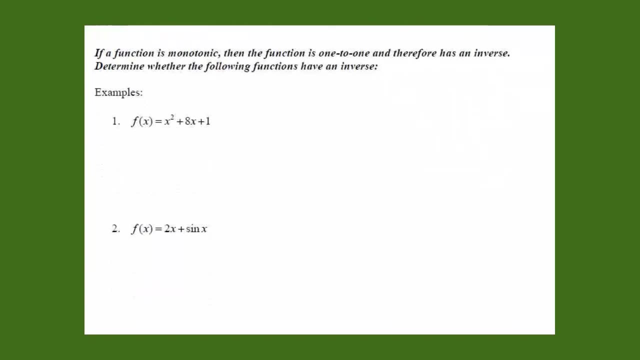 And that would imply that a function has it is monotonic, which means it does have an inverse and it is 1 to 1.. Okay, so we're going to look at some examples here. These are in your notes handouts. It says that if a function is monotonic, then the function is 1 to 1 and therefore has an inverse. So we're supposed to determine whether the following functions have an inverse: 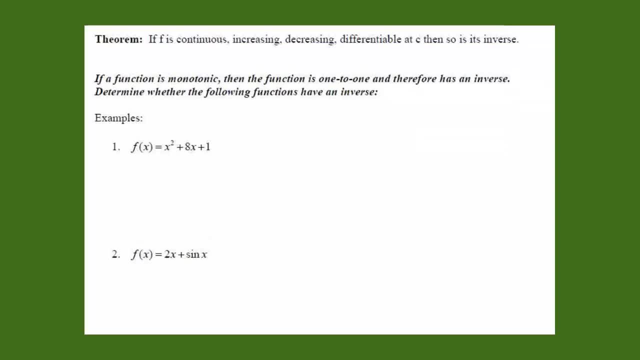 Okay, so we're just going to use our property, that our theorem, that just says: if our function is monotonic, then yes, It is 1 to 1 and yes, it does have an inverse. So that means, in order to do this, we can just find the derivative for each of these and test the derivative to see if it is always positive or always negative. 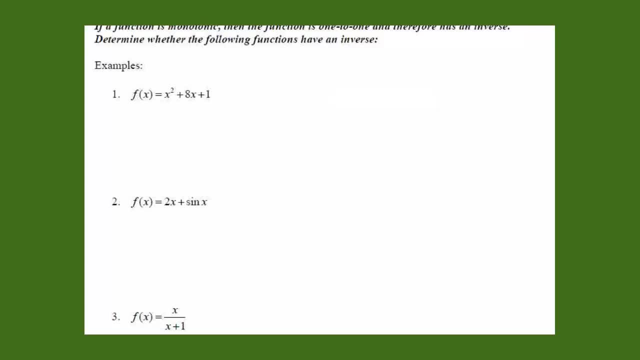 And if yes, then that means that our function does have an inverse. Okay, rather than trying to go and actually find the inverse Okay. so for example number 1 we have: f of x is equal to x squared plus 8x plus 1.. 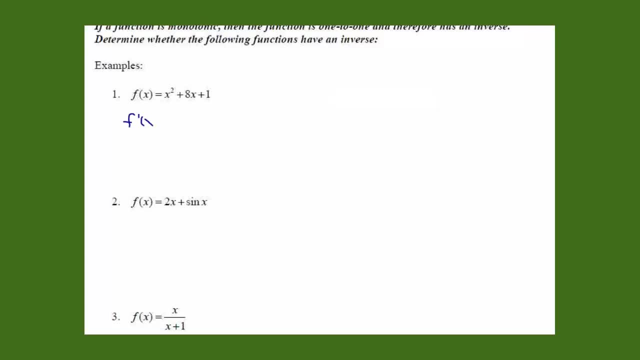 So the first thing we'll do is we'll go ahead. We can get a derivative, so f prime is equal to 2x plus 8, and we'll go ahead and set the derivative equal to 0, and when we do that we get that x is equal to negative 4.. 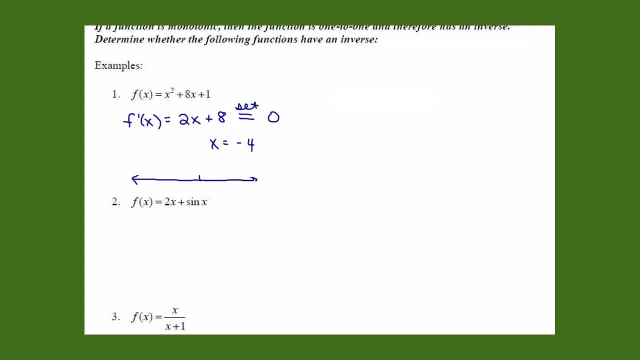 Okay. so then we want to test this critical number: x equals negative 4.. We want to test f prime and we want to see what is the sign for f prime. So if we plug in numbers smaller than negative 4.. So, for example, negative 5 and 4 f of x, we get a negative number. 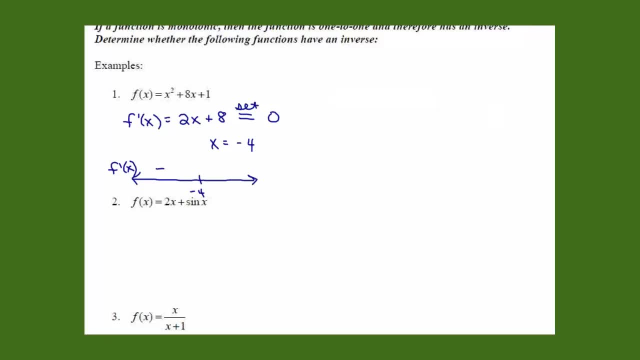 But then when we plug in numbers larger than negative- 4, so like 0 and 4 f prime- we get a positive number. Okay, so here, this derivative tells us that our derivative sign changes from a negative to positive, which implies that we have a turn in the graph. 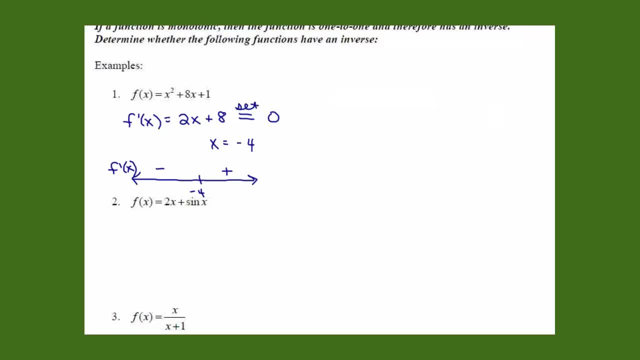 So that means that it's not monotonic, It's not 1 to 1, so there is no inverse function. So not monotonic, Not 1 to 1.. No inverse. This is all because f prime changes signs. Now, if they wanted to restrict the domain, 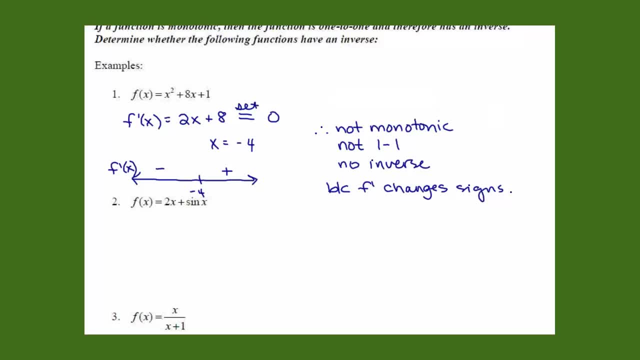 So, for example, if they said: on the interval from negative 4 to infinity, does this function have an inverse? Well, there we would be able to answer yes, because the derivative would be positive for all of those values. But on the interval from negative infinity to positive infinity, no, there is not an inverse function. 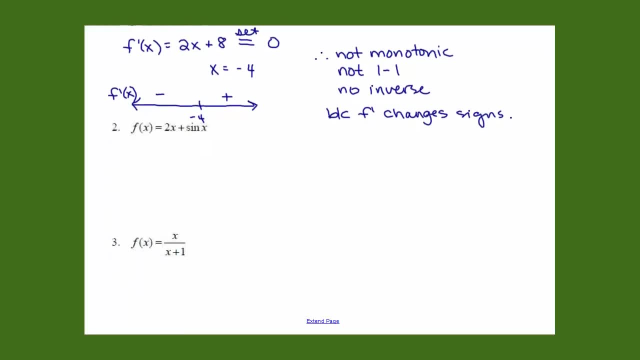 Okay, example 2: we have: f of x is equal to 2x plus sine of x. Okay, so same question. We want to know: Does this function have an inverse? So we're going to go ahead and take a derivative. So f prime here will be 2 plus cosine x. 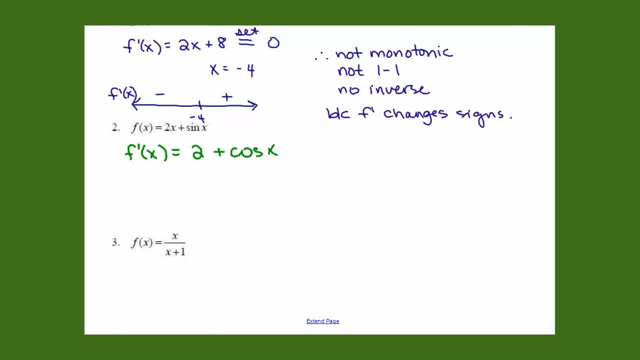 And when you look at the function of 2 plus cosine x, you don't even necessarily have to find a critical number or do any kind of sign chart business, because if you just look at cosine of x, you know those values are going to be positive. 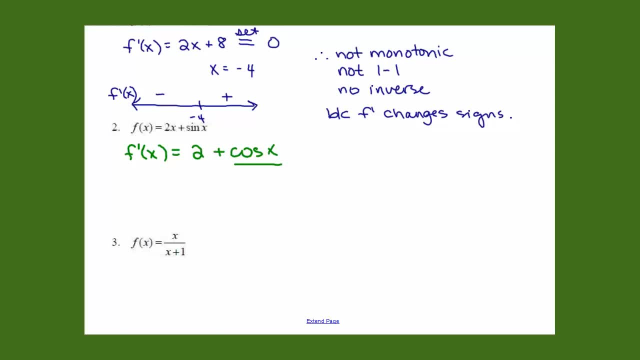 Okay, So that's going to be negative 1-1.. So if you add 2 to that, That whole graph has now been shifted above the x-axis. So this is greater than 0 for all x, And so that means that, yes, we would have an inverse. 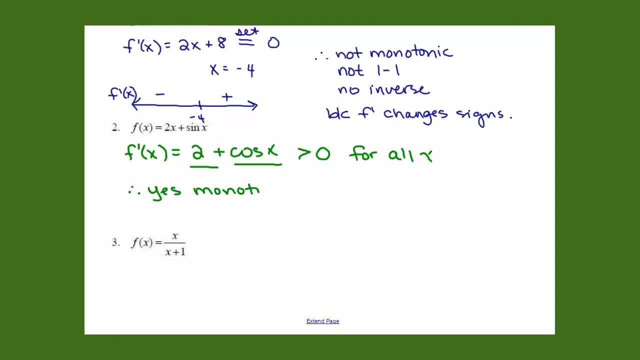 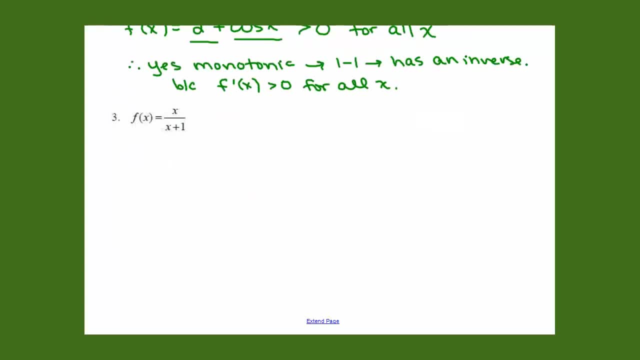 okay, example 3: okay, same question. we have f of X is equal to X over X plus 1, and we want to know whether or not this is a monotonic function. therefore one to one and having an inverse, okay, so we'll go ahead and take the derivative. so 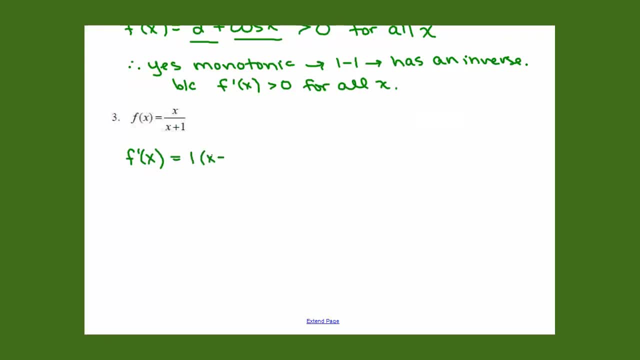 using the quotient rule, we need the derivative of X times X plus 1 minus X times the derivative of X plus 1, all over X plus 1 quantity squared, and this will just simplify to 1 over X plus 1 quantity squared. okay, so the only. 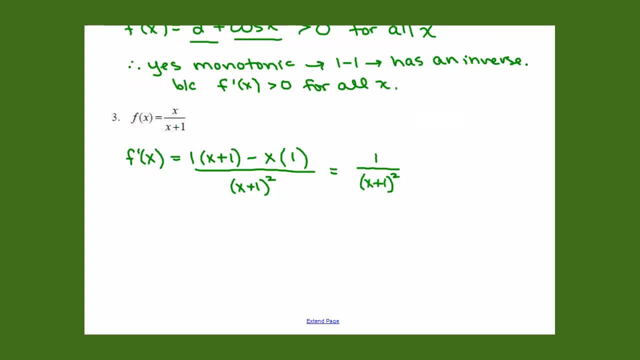 critical numbers for this derivative is when X is equal to negative 1 coming from the denominator. so when we test X is equal to negative 1 into f prime if we plug in numbers to the left of negative 1, so like a negative 2 plug. 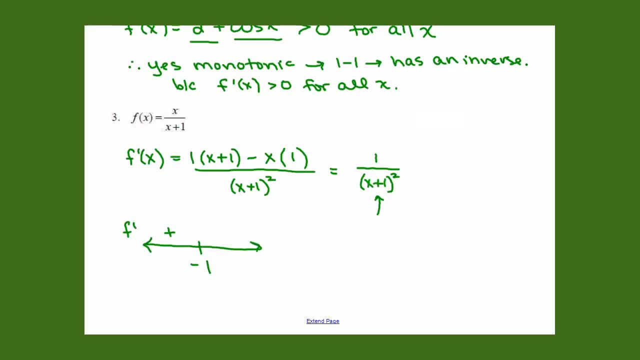 that into our derivative function we get a positive value. if we plug in numbers larger than negative, 1 into our derivative function, so, for example, 0, we get another positive value. so our derivative goes positive. positive, it's always a positive function value for our derivative. so this is: 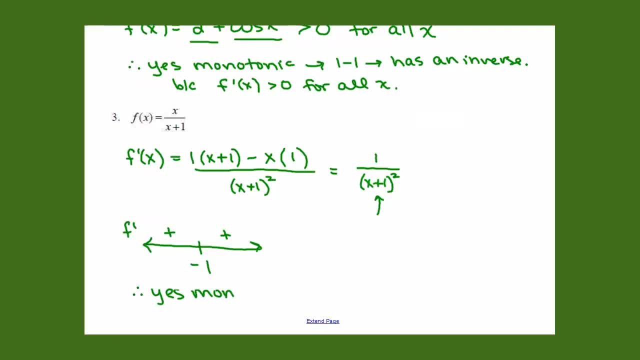 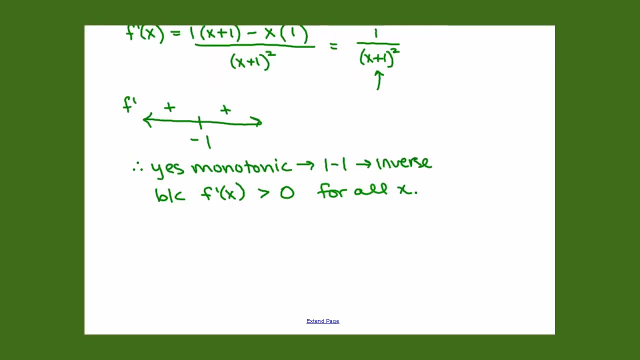 another yes. so, yes, it's monotonic. so that means it's 1 to 1, which means there's an inverse, because f prime of X is greater than 0 for all X. okay, so that's it for the monotonic functions. the next video, then you'll be learning how to take. 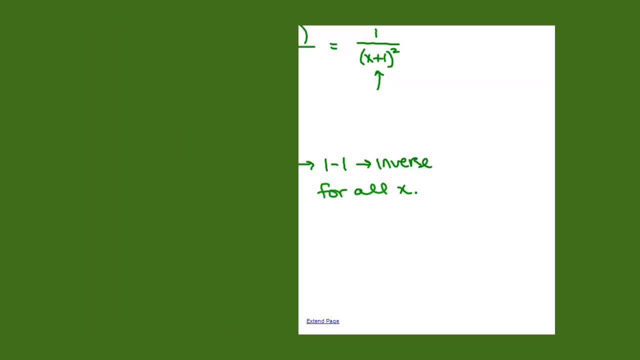 derivatives of inverse functions. so we'll. see you then.